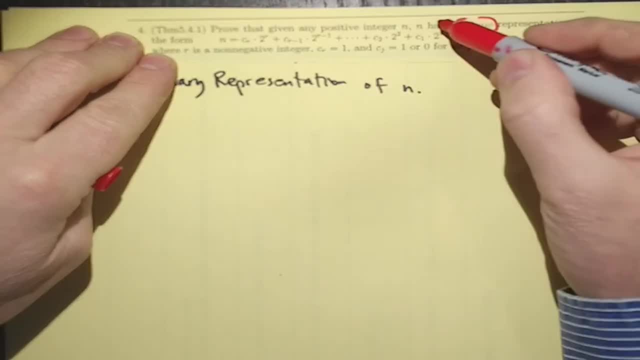 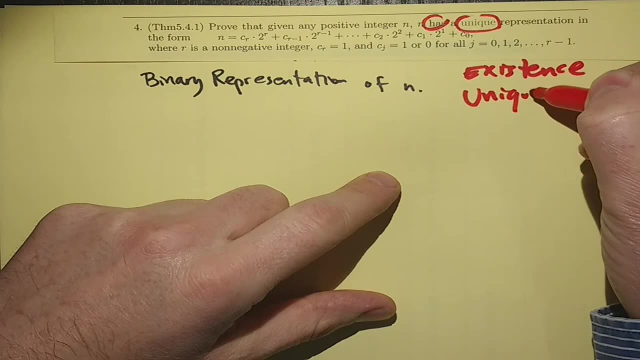 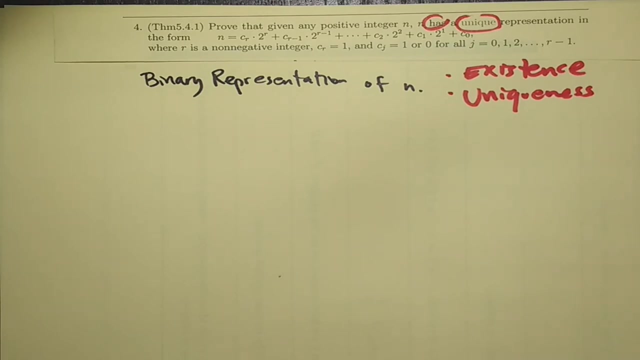 There's a there's existence and there's uniqueness, And those are actually things that are better proven separately: Existence and uniqueness. Now, let's do, let's do existence, Let's start with existence, and then we'll follow up by uniqueness. 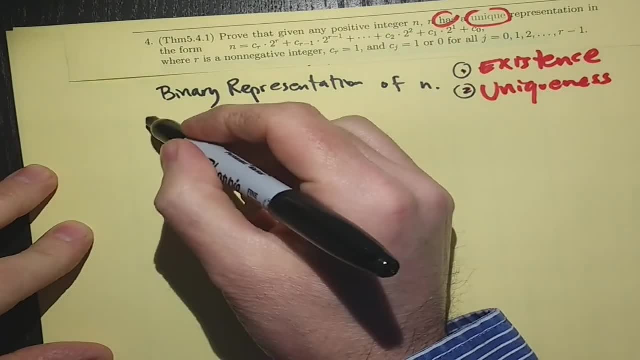 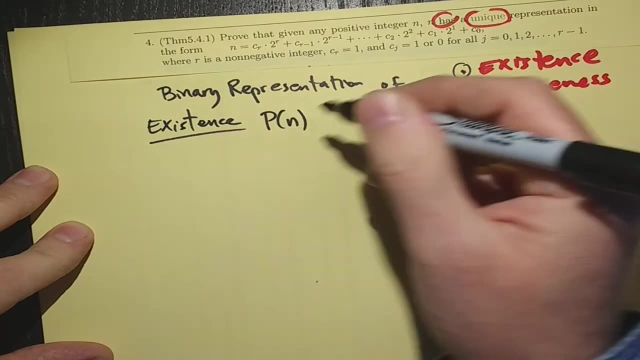 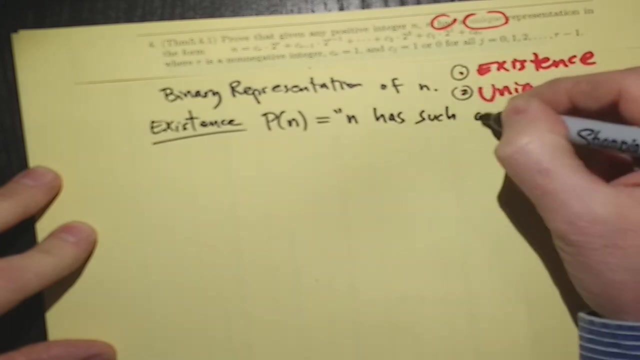 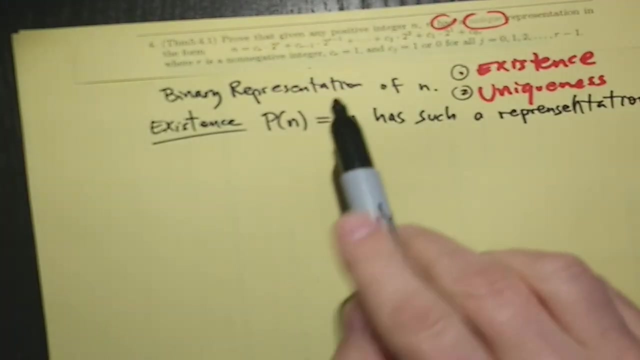 For existence, existence, existence, existence. I'll use strong induction, existence, and my statement p of n is going to be the statement n has such a representation: Represen, represent, representation. Okay, here we go, And that's how it's written. Each of the bits is 1 or 0.. 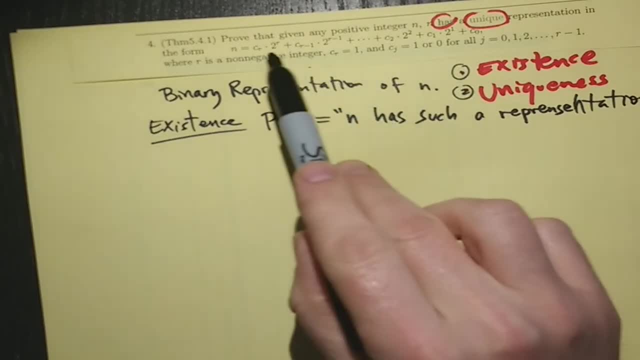 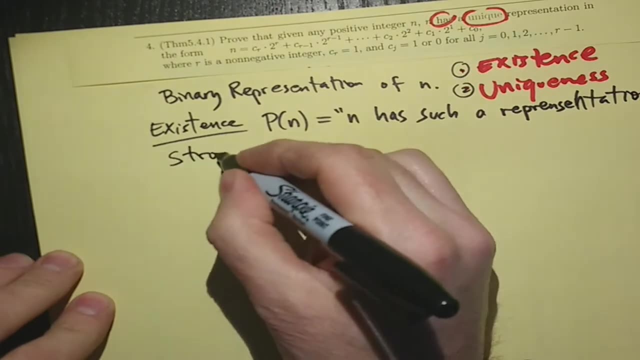 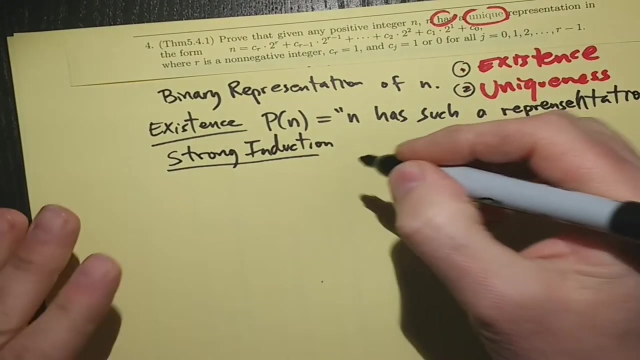 The first one has to be a 1, and we have decreasing powers of 2.. We'll be using strong induction And let's forget about the base case. If you want a base case, you could say that p of 1,. 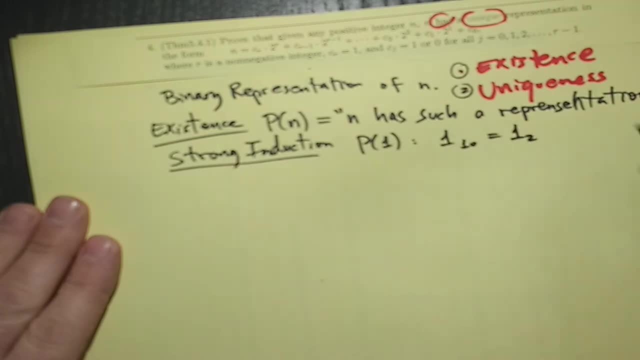 1 in base 2 is 1.. 1 base 10 is 1 base 2.. If we want another base, case 2 base 10 is 1, 0 base 2.. So this is 1 times 2 to the 0.. 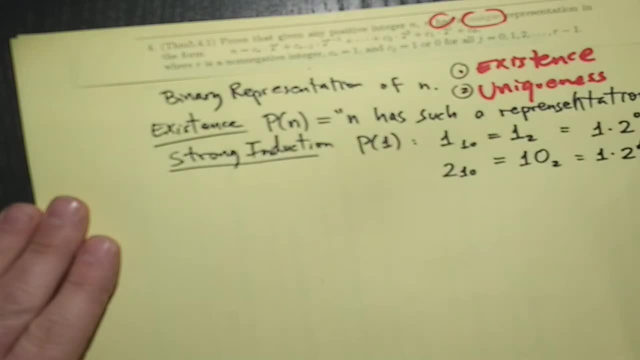 Over here. this is 1 times 2 to the 1 plus 0 times 2 to the 0, and so on. So you could just start writing out the binary representation for any of these numbers. But let's do the induction step. 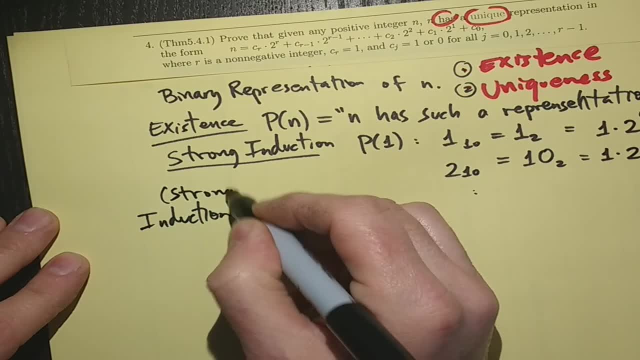 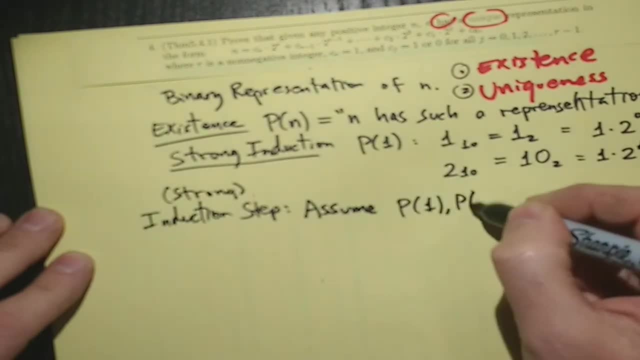 And of course it's going to be a strong induction step. So we're going to assume that p of 1, p of 2, all the way up to p of k are true. That just means that every number from 1 to k has a binary representation. 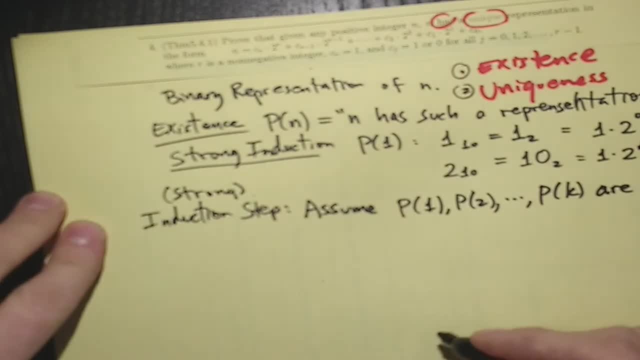 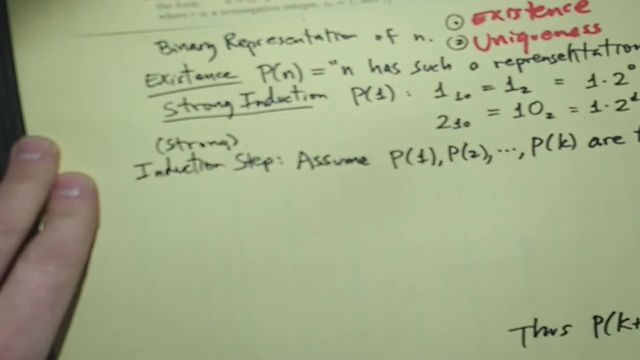 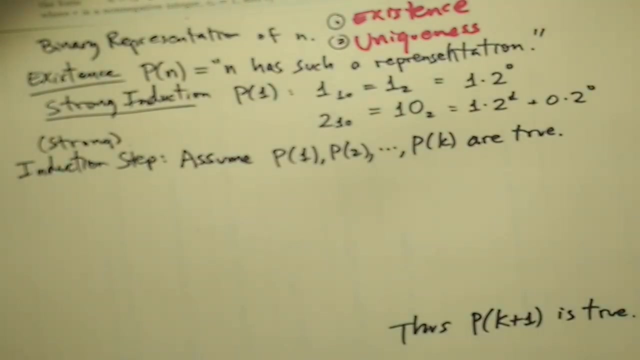 And we'd like to conclude that p of k plus 1 is true as well. So that's what we need to do, And it's not going to be hard: We're going to assume that every number less than k plus 1 has a binary representation. 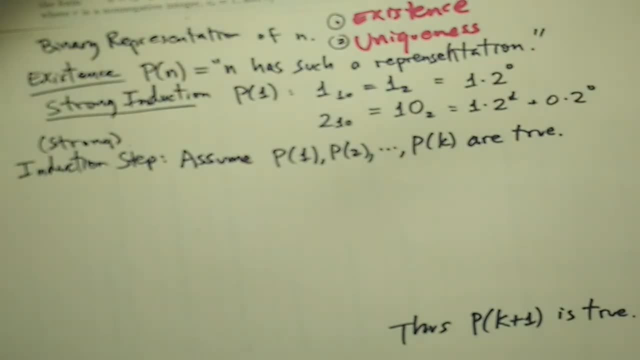 And we'll prove that k plus 1 also has a binary representation. So here we go, And I'm going to write this in two cases. Let's call them case even, And the other will be case odd, And k plus 1 is. 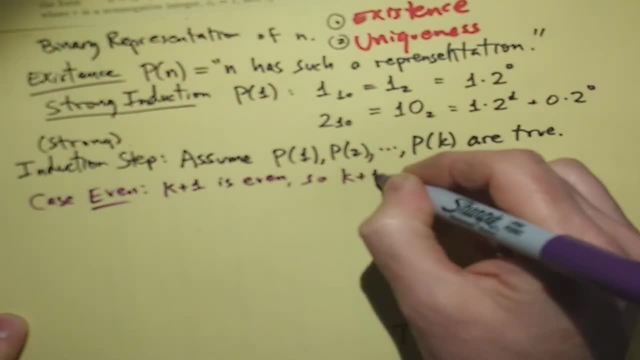 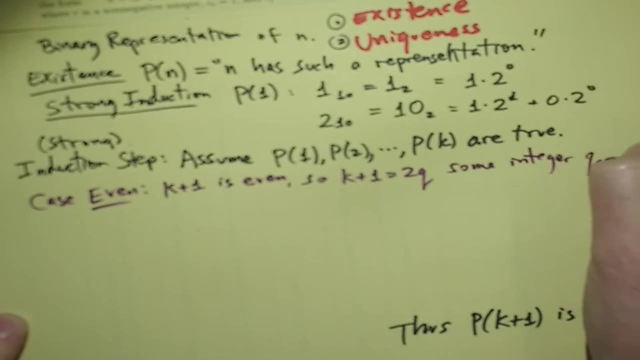 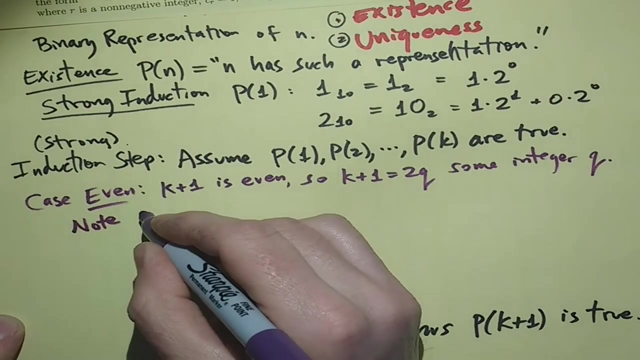 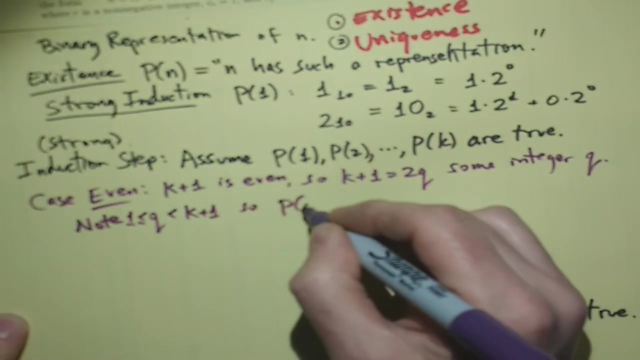 Even So, k plus 1 is 2 times q And that's some integer q. And I'd like to note that q is at least 1, and it's less than k plus 1.. So p of q is true. 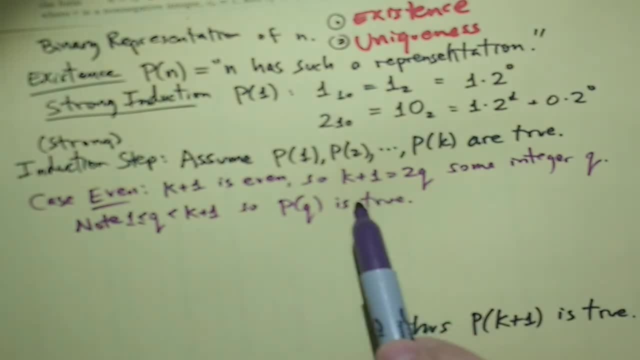 Why is that? Well, maybe I could go into more detail. But if k plus 1 is twice q, then q must be less than k plus 1. And q is also going to be at least 1.. So p of q is true. 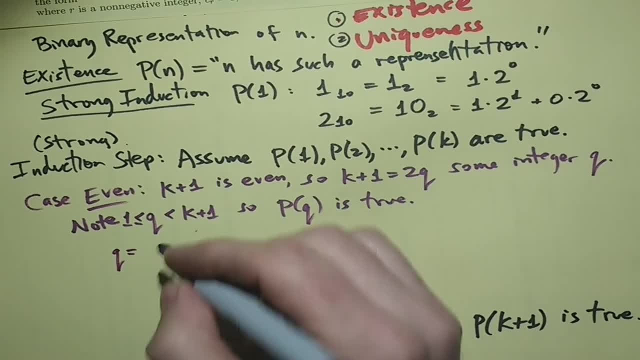 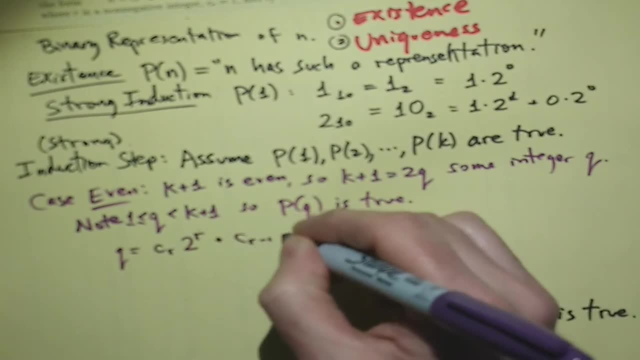 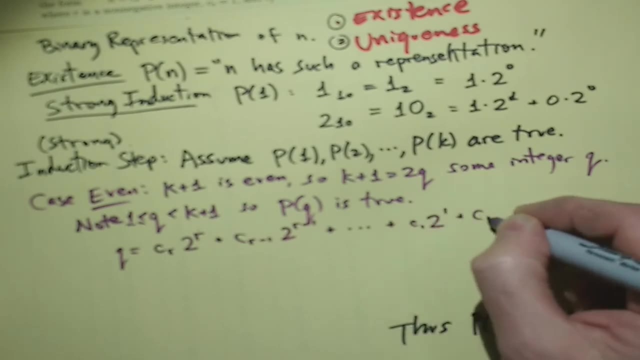 That means that q does equal cr2 to the r plus cr minus 1.. 2 to the r minus 1 plus all the way down to c1. 2 to the 1 plus c0, for some binary digit cr down to c0.. 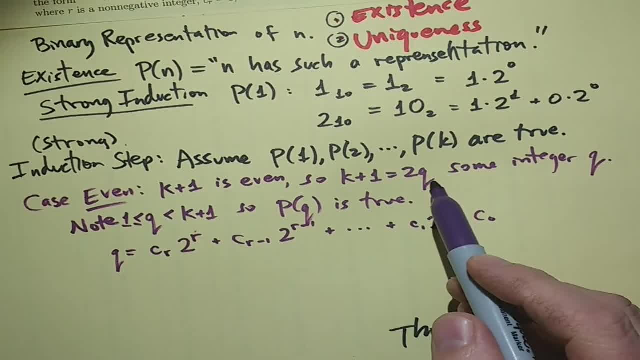 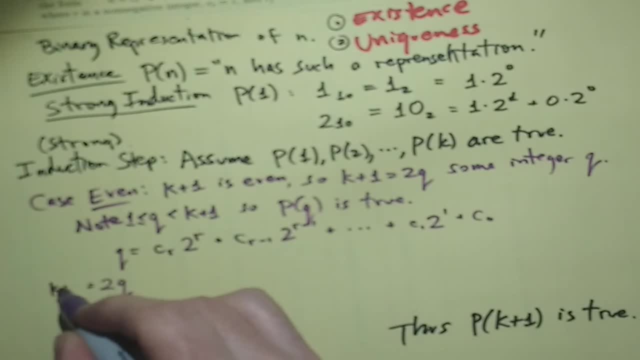 And those are the powers of 2.. But now, when we multiply it by 2, 2q- which, by the way, is k plus 1, that's k plus 1, that's going to equal cr2 to the r plus 1 plus cr minus 1, 2 to the r plus 1.. 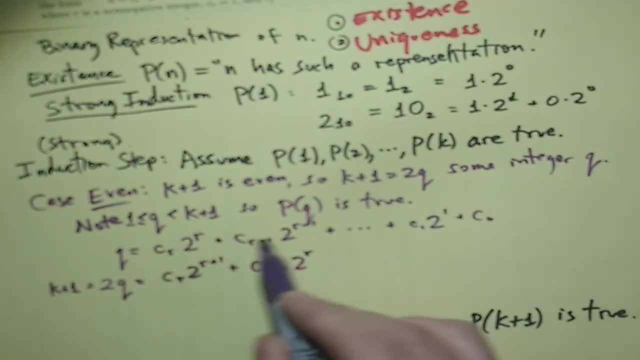 2 to the r minus 1.. 2 to the r minus 1. 2 to the r, Because we're multiplying everything by 2, I could multiply 2 to the r times 2 to get 2 to the r plus 1, and so on. 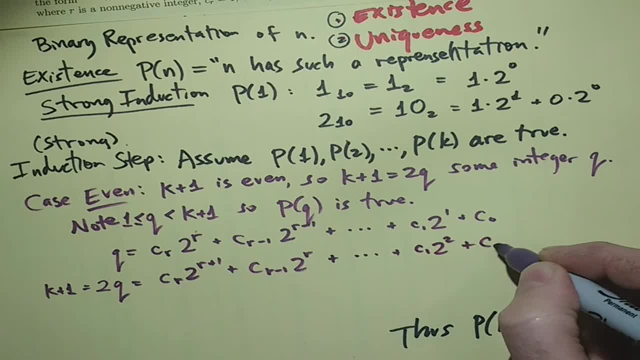 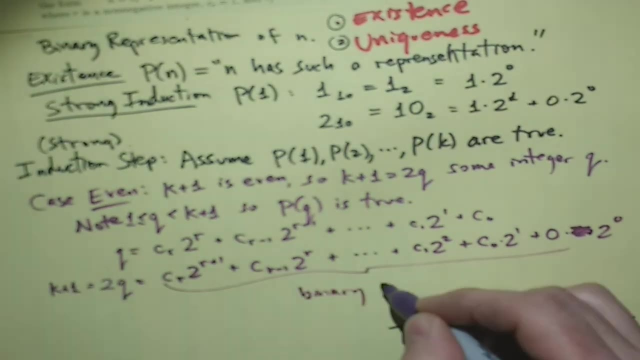 And c1, 2 squared plus c0 times 2 to the 1, plus a 0 times c, well, times 2 to the 0.. And so, all of these, this is a binary representation, a binary representation for k plus 1.. 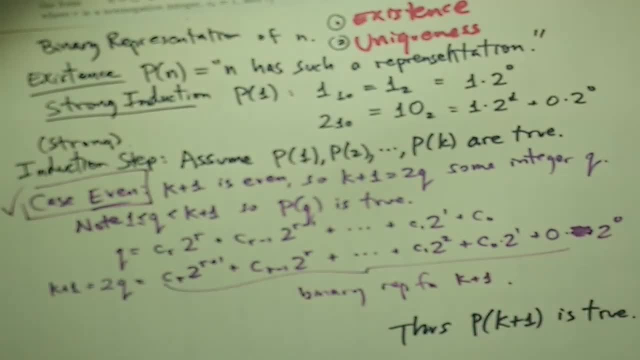 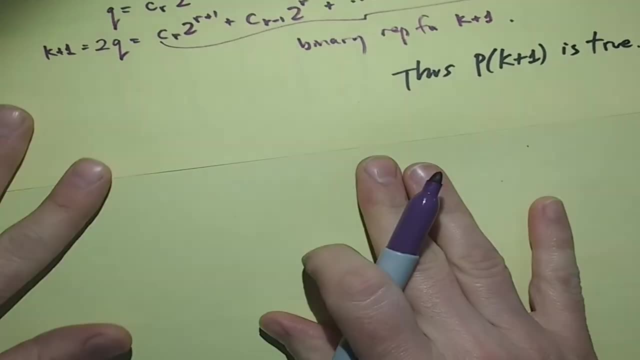 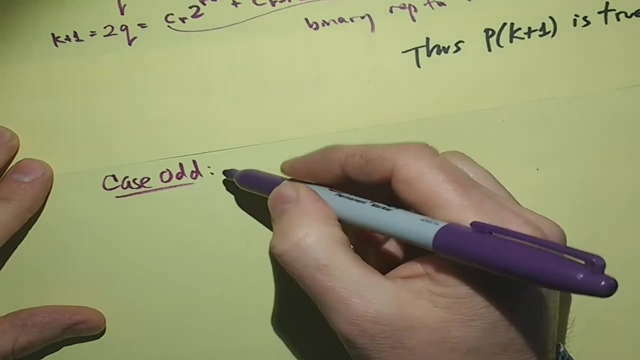 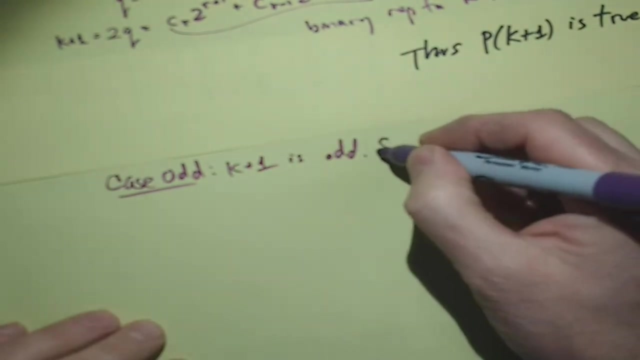 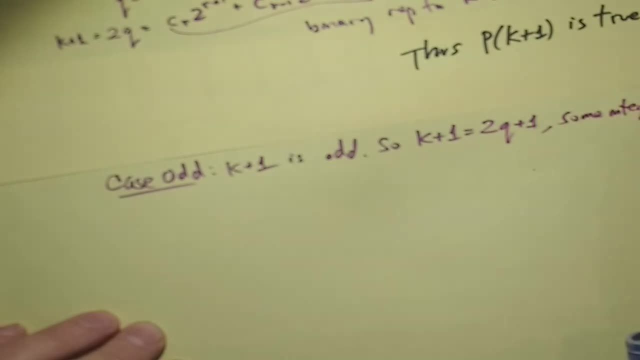 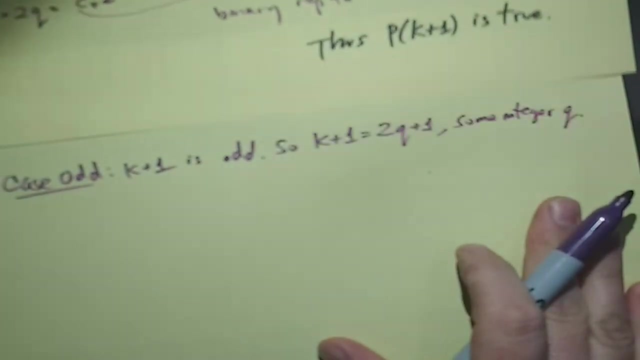 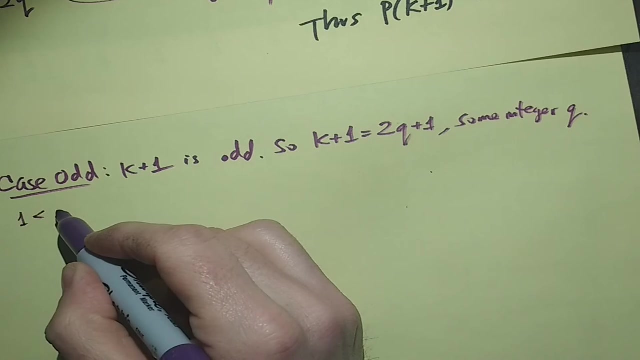 2q plus 1.. For some integer q, For some integer q, That means that well, let's see if we can do this. q is less than k plus 1.. If k plus 1 is 2q plus 1, then k is 2q. 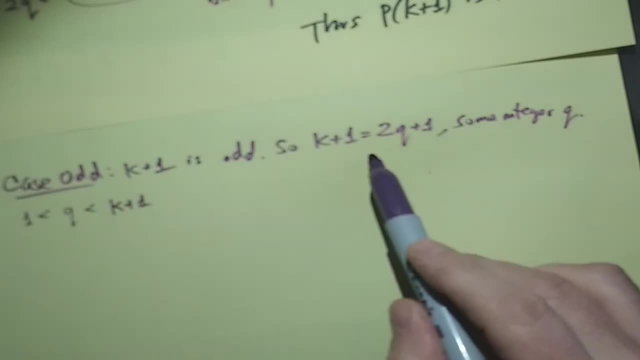 2q. That means that k is bigger than q, but k is odd, So k plus 1 will be even bigger And we can assume that q is well, q is q might actually be 0.. Maybe that's a special case. 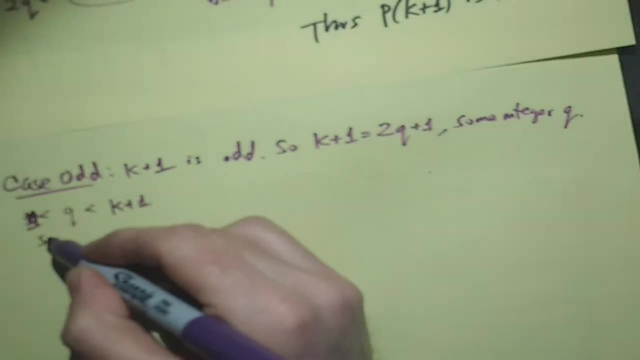 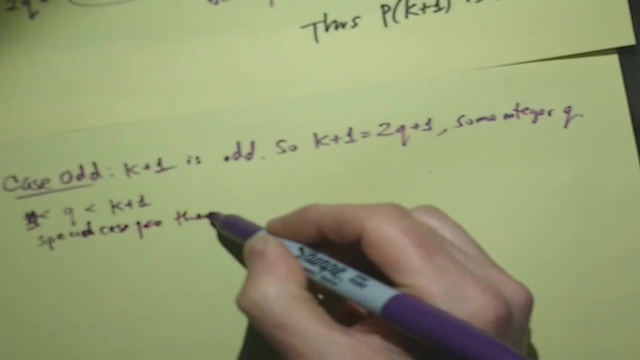 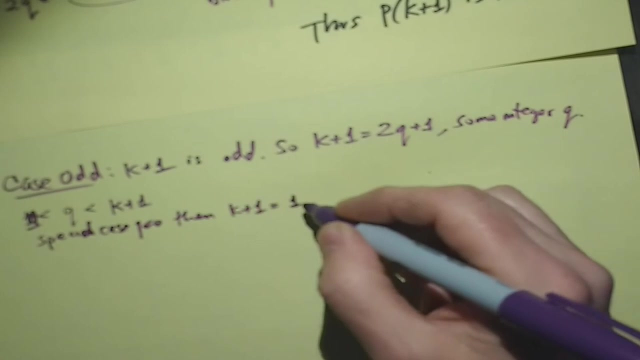 Yeah, so let's have a special case. Yeah, so let's have a special case. q equals 0. Then k plus 1 is k plus 1 is 1, which is 1 and base 2.. So let's forget about that.